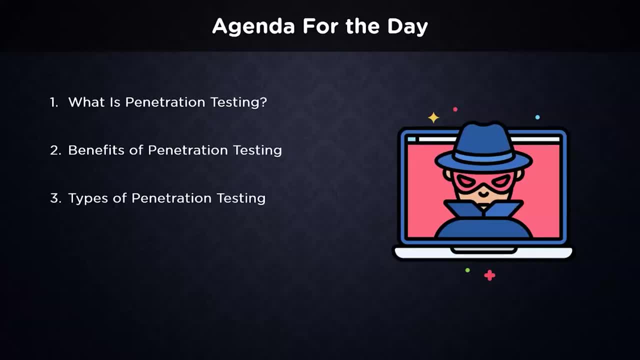 and the benefits of penetration testing. Next, we know about the benefits of penetration testing and the benefits of penetration testing. Next, we know about the benefits of penetration testing and how they help organizations save money in the long run. Moving on, we familiarize ourselves. 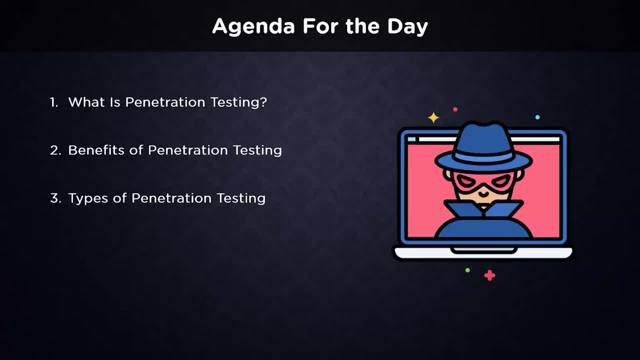 with the different types of penetration, testing or ethical hacking, with each serving a different category of personnel. In the next section we read about the five distinct phases in every ethical hacking campaign and how they help clear up the extensive report at the end of every. 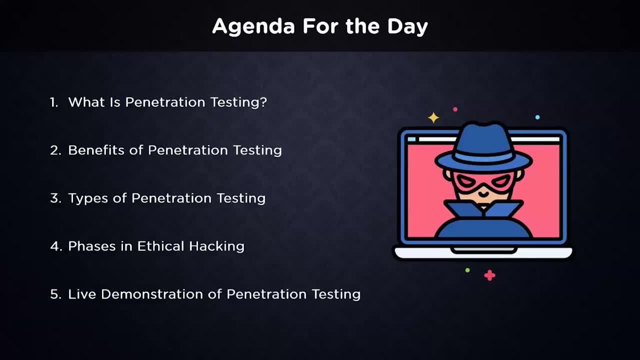 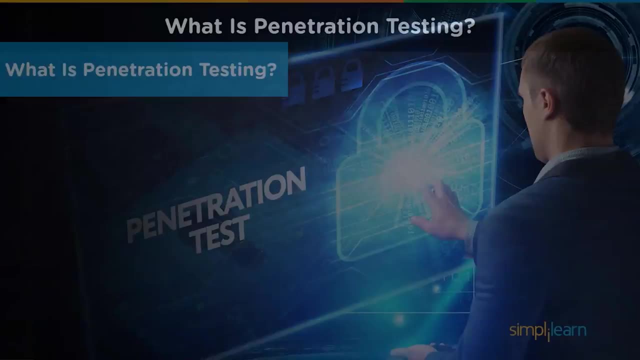 penetration testing session. Finally, we have a live demonstration on how we can check for vulnerabilities and the ways hackers can break into a device and use it to hack. Let's start by learning about penetration testing in general. Organizations can define penetration testing based on the objectives of the test. 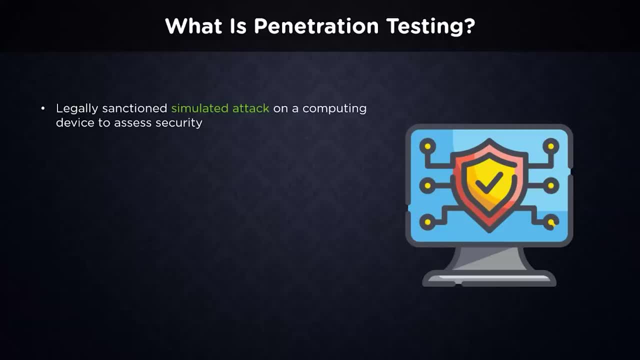 All networks, applications, devices and physical security components are included. It imitates the behavior of harmful individuals or the hackers. Experienced cybersecurity specialists use penetration testing to strengthen a company's security posture and eliminate any weaknesses that leave it vulnerable to attacks. 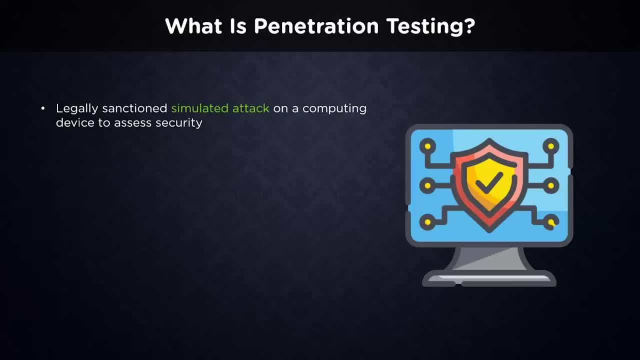 Penetration testing, when done correctly, goes beyond simply preventing thieves from gaining unauthorized access to a company's systems. It generates realistic scenarios that demonstrate how well a company's present defenses might perform in the face of a full-scale cyber-assault. The simulation aids in the discovery of the sites of exploitation and 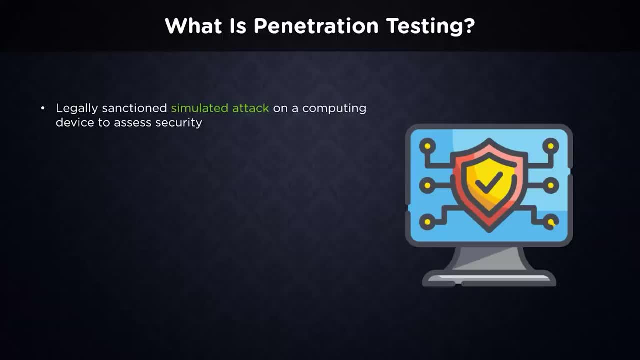 the testing of IT breach security, Businesses may acquire professional, unbiased third-party input on the security process. They may also be able to access the security of the company through the procedures by conducting frequent penetration testing. Penetration testing, while relatively time-consuming and costly, can aid in the prevention of highly destructive and expensive 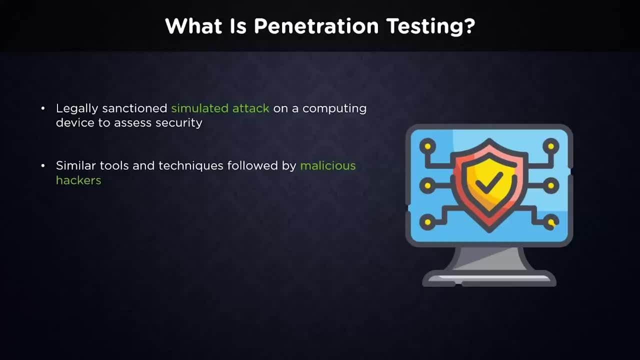 breaches. A white hat hacker employs hacking talents to find security flaws in hardware, software or networks. On the other hand, white hat hackers follow the rule of law when it comes to hacking. instead of black hat hackers, They assist firms in conducting penetration tests to analyze their security index and make the necessary improvements. 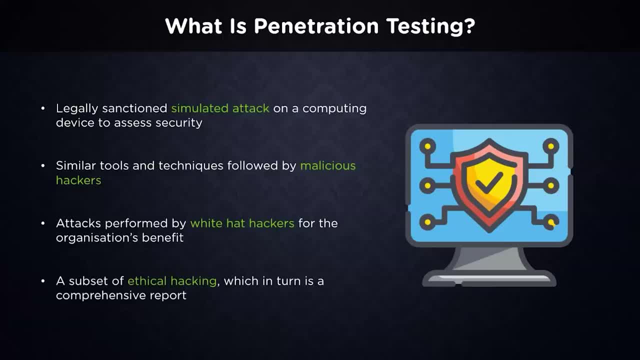 Ethical hacking provides a full audit of your security policies and, in the case of bug bounties, can assist you in identifying holes in existing operational systems. It takes a far broader approach to cybersecurity than penetration testing. Whereas penetration testing focuses on system flaws, ethical hacking allows actors to utilize any attack tactics available to them. 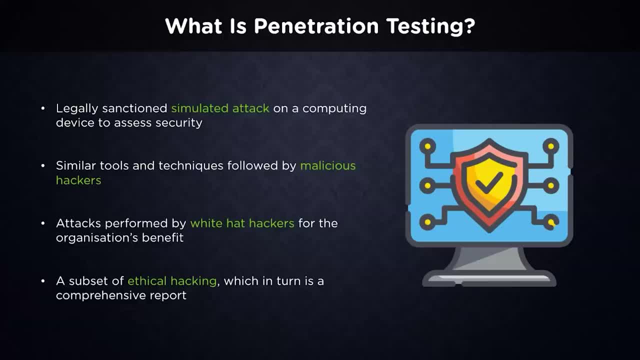 They can take advantage of system misconfigurations, send phishing emails, launch brute-force password assaults, breach fraud and more. They can take advantage of system misconfigurations, send phishing emails, launch brute-force password assaults, breach fraud and breach physical boundaries, or do whatever else they feel will get them access to critical. 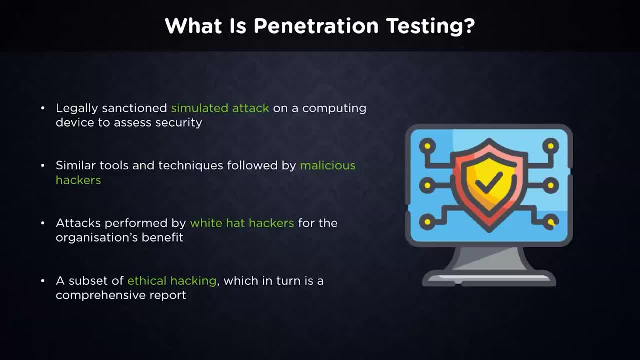 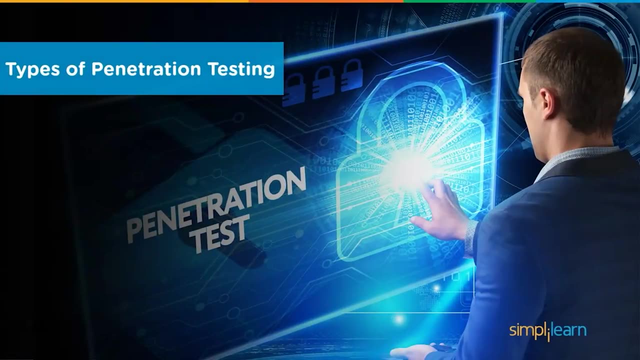 information, Because thieves are progressively changing approaches and launching multi-layered, complex attacks. this is incredibly useful for determining just how exposed the organization is to cyber threats. Considering the vast domain that is ethical hacking, we have multiple categories of penetration testing methodologies. Let's cover them in the next section. 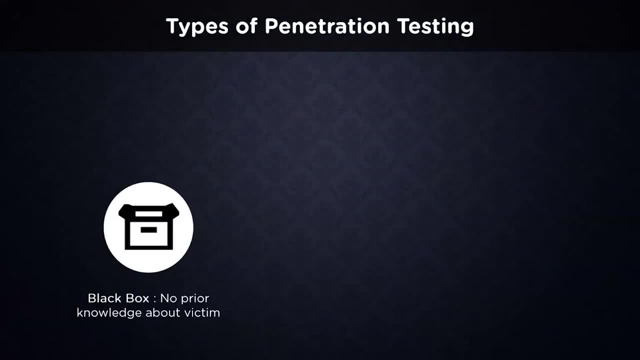 When configuring a security system, testing is critical to preventing hackers from penetrating the perimeter. There are three sorts of tests: black box, gray box and white box. In the black box testing, the tester receives no information during the penetration test. In this case, the pentester takes the method of an unprivileged 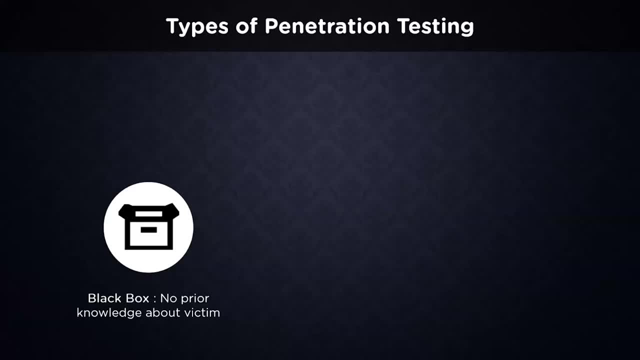 attacker from initial access and execution until exploitation. This scenario is the most realistic, showcasing how an attacker with no inside knowledge may target and compromise an organization. However, because of this, it is also the most expensive alternative. White box penetration testing, which is also known as crystal box testing. 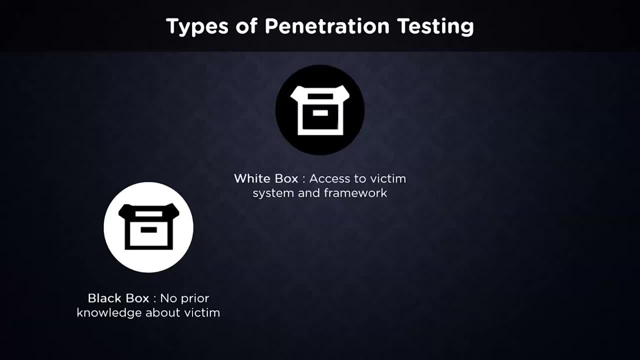 entails sharing all network and system information with the tester, which includes network maps and passwords. This saves time and lowers the overall cost of a project. A white box penetration test effectively simulates a focused assault on a given system using as many attack paths as feasible. 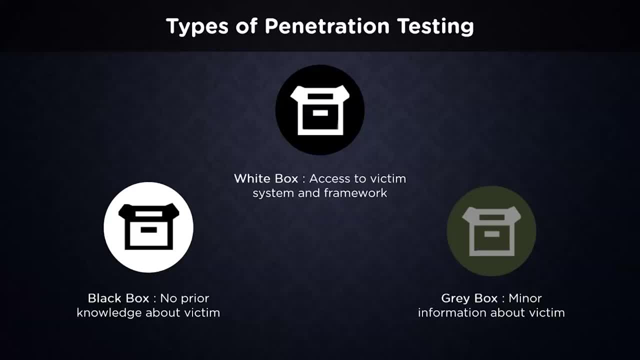 In a gray box penetration test, also known as a transparent box test, very restricted information is shared with the tester. Gray box testing is beneficial for understanding the extent of access a privileged person may get and the possible damage they could wreak. Gray box test. 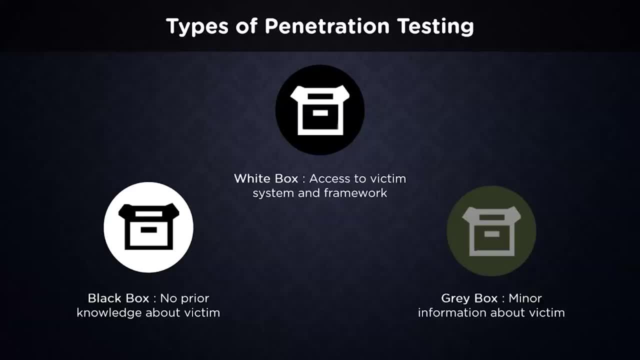 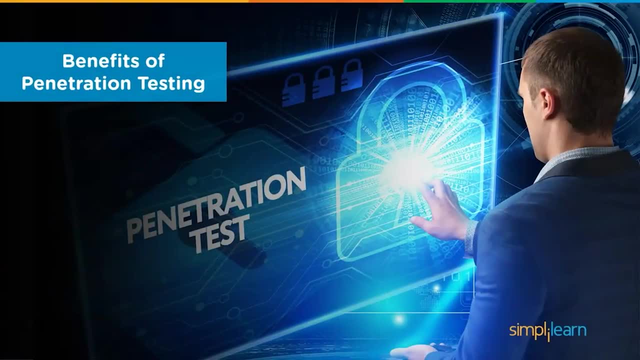 achieve a mix between depth and efficiency, and may be used to mimic either an insider danger or an assault that has infiltrated the network perimeter. Now that we covered the basics of penetration testing and their relative categories, one must know how these testing campaigns benefit the organizations conducting them. 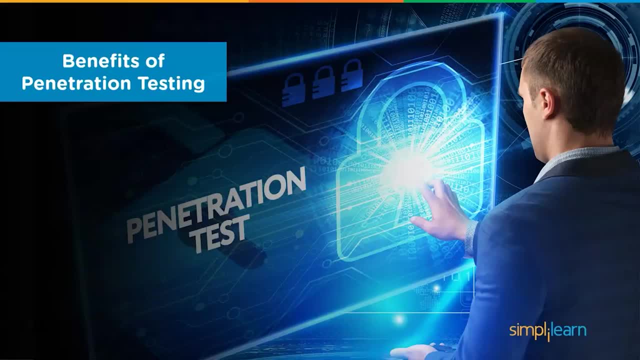 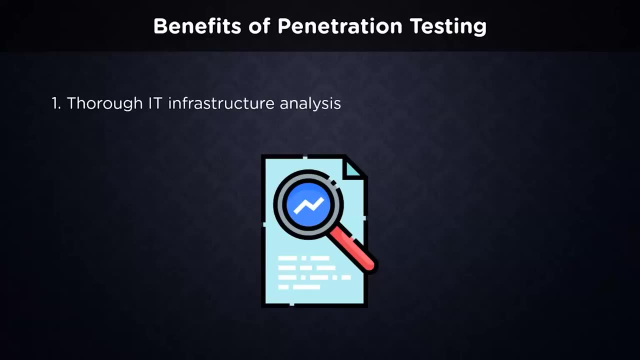 Let us go through a few perks of penetration testing. Regular penetration testing helps your business assess the security of online applications, internal networks and external networks. It also assists you in understanding what security measures are required to achieve the degree of protection your company needs to protect. 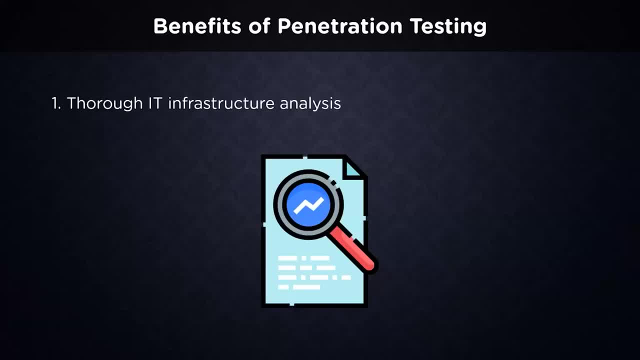 its people and assets. Prioritizing these risks offer firms an advantage in anticipating hazards and preventing harmful assaults. Penetration testing is similar to a real-life hacker rehearsing for a real-life hack. Regular penetration testing helps you be proactive in your real-world approach. 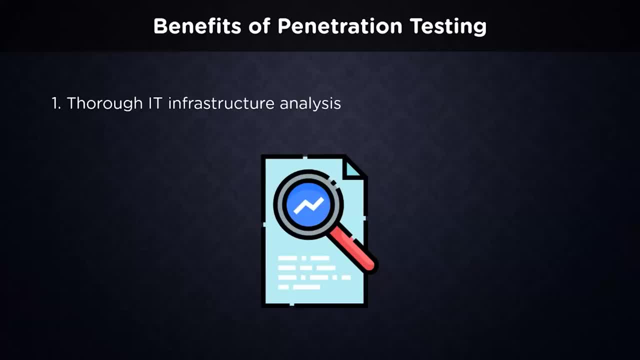 to reviewing the security of your IT infrastructure. The process identifies gaps in your security, allowing you to correct any flaws before an actual attack happens. It is undeniably expensive to recover from the effects of a data breach: Legal fees, IT cleanup. 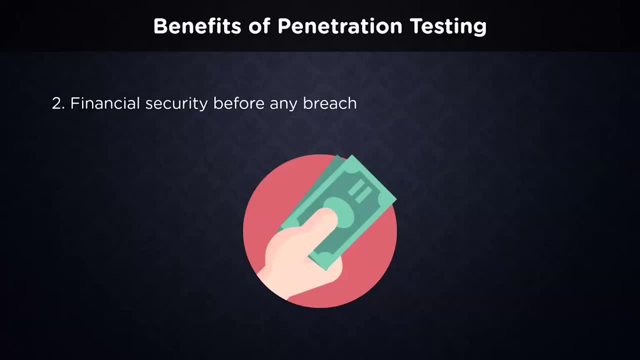 consumer protection programs lost revenue and dissatisfied customers. It is also expensive to recover from the effects of a data breach. Penetration testing regularly is a proactive strategy to remain on top of your security and may assist in preventing financial damage from a breach while safeguarding your brand and image. Penetration testing aid in meeting the compliance. 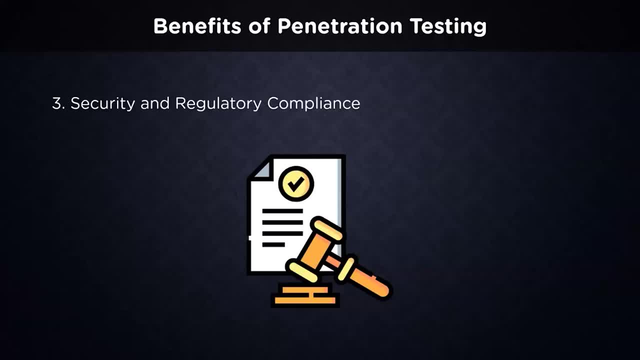 and security duties imposed by industry standards and regulations such as PCI, HIPAA, FISMA and ISO 27001.. Having these tests done regularly help demonstrate due care and your commitment to information security, all while avoiding the significant fines associated with the non-compliance. 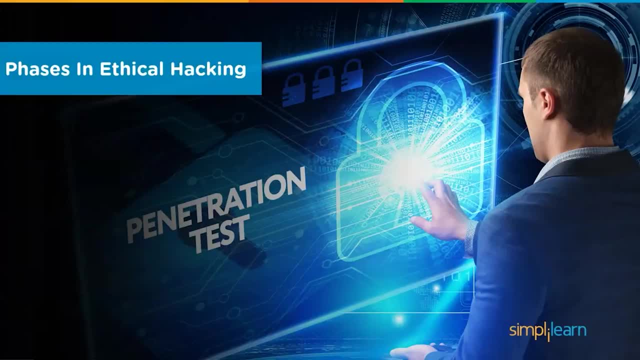 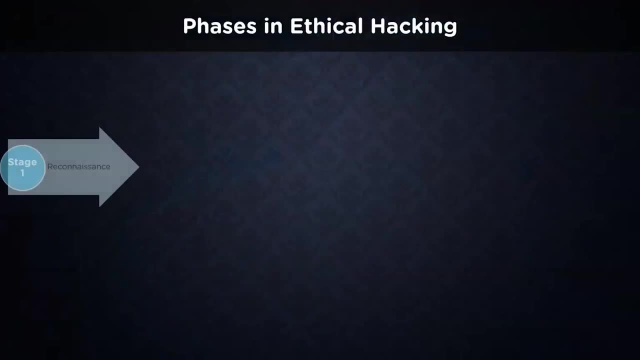 With the entire process seeming to be a lengthy ordeal. what are the multiple phases in the process? Theoretically, we have to follow a five-stage process. Reconnaissance is the first phase of the penetration test. In this phase, the security researcher collects information about your target. It can be done actively, meaning you are collecting. 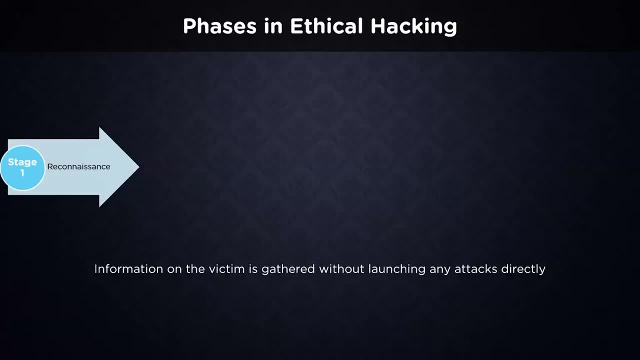 information by sending a request directly to the target and interpreting it passively, whether you are collecting data without contacting the target or both. It helps security firms gather information about the target system, network components, active machines, etc. This activity can be performed by using information available in the public domain and using different tools. 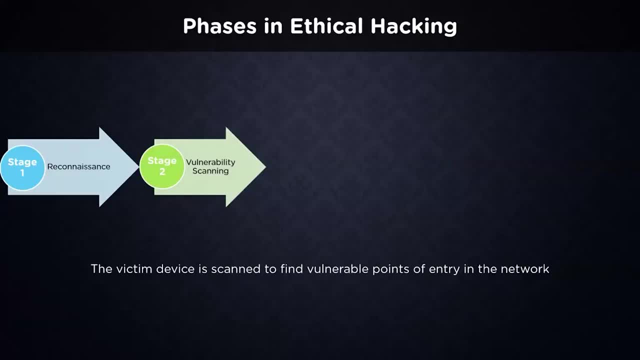 The scanning phase is more tool-oriented rather than performed manually. The penetration tester runs one or more scanner tools to gather more information about the target By using scanners such as ward dialers, port scanners, network mappers and vulnerability scanners. the penetration 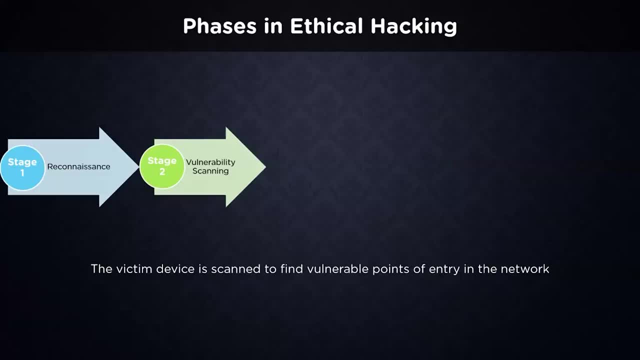 tester collects as many vulnerabilities which help in turning to attack a target in a more sophisticated way. The third phase is gaining access of the system. In this phase, the penetration tester tries to connect with the target and exploit the vulnerabilities found in the previous stage. 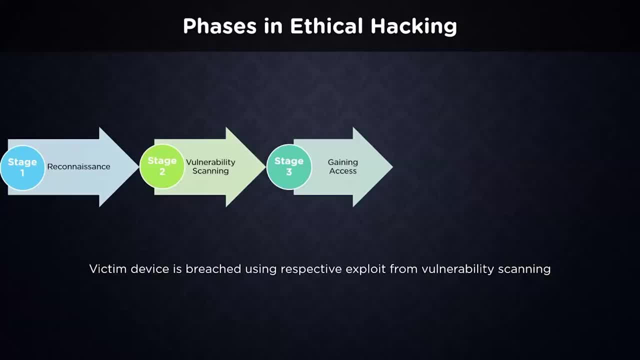 The penetration may be buffered over flow attacks, denial of service, DOS attacks, session hijacking and many more. The penetration tester extracts information and sensitive data from the servers by gaining access using different tools. In the fourth stage, the hacker helps to maintain. 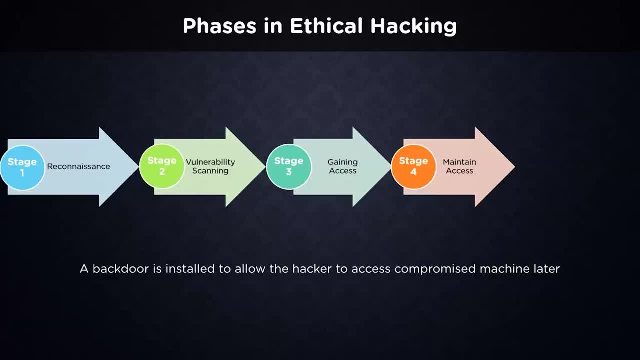 access. The penetration tester tries to create a backdoor for himself. It helps the penetration tester to identify hidden vulnerabilities in the system and can later access the machine should the need arise. In the final phase of clearing and covering tracks, the penetration tester removes all. 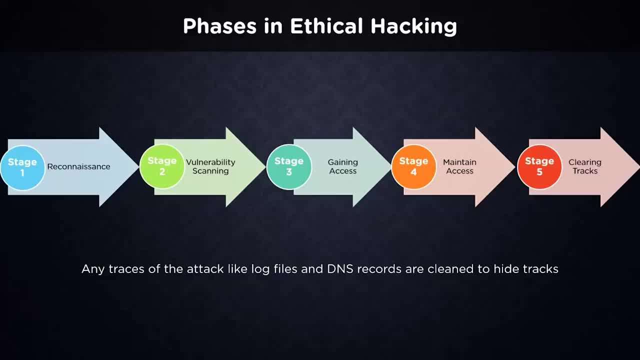 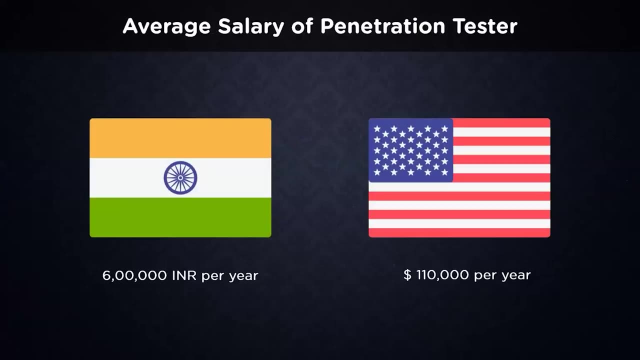 logs and footprints which help the administrator identify his presence. This allows the penetration tester to think like a hacker and perform corrective actions to mitigate those activities. With the cost of cybersecurity platforms going up, trained penetration testers receive an excellent level of remuneration for their efforts. 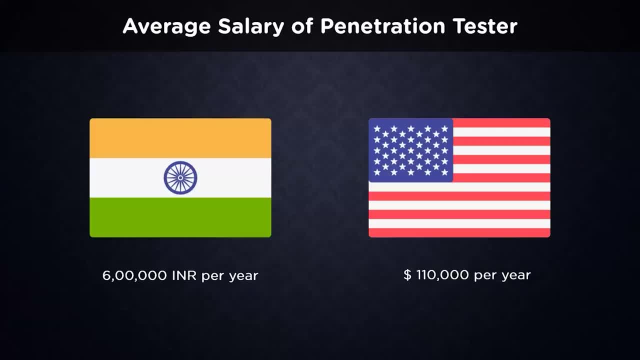 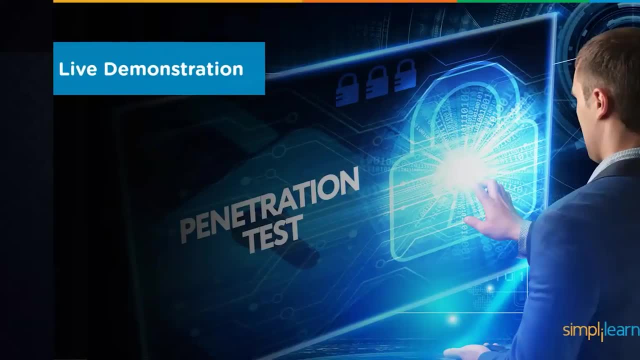 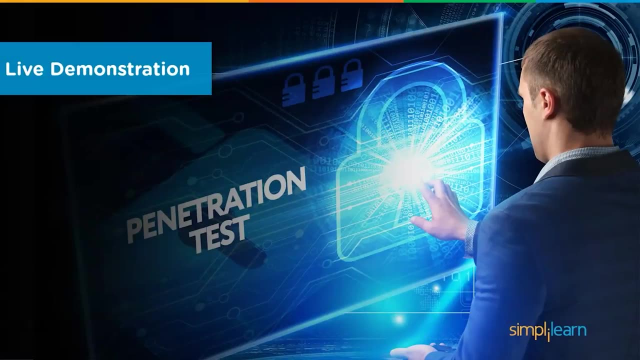 As per reports, the average yearly salary for a penetration tester is 6 lakh Indian rupees, or 100- 10 thousand dollars in the American counterpart. Finally, let's go over some of the ways hackers can identify vulnerable positions on a system to gather information in a live demonstration. 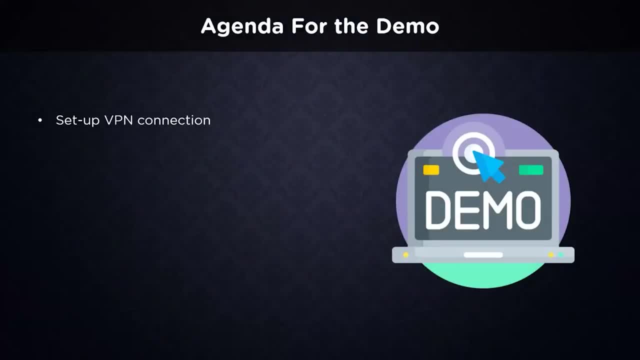 In this demo, we will start by setting up a VPN connection that will allow us to access to a vulnerable network by creating a local virtual group over the internet. We then try to scan the victim machine for breachable entry points, find the username and password of the user in question. 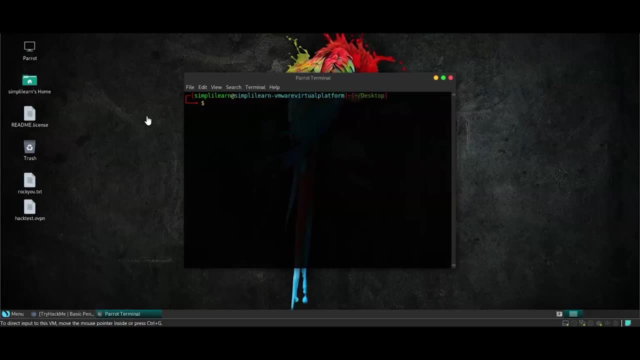 and eventually grab the root password from the device To start our demonstration. we're going to need a vulnerable machine to work on Now. this vulnerable machine can be found on the website known as TryHackMe, which is a service catered towards penetration testers. Before we connect to the machine, we need to join the network. 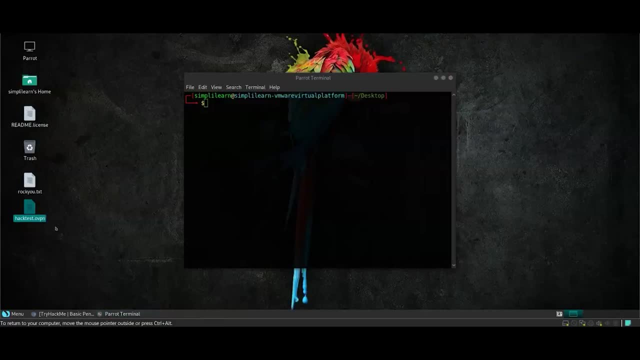 where the machine is located. We can do that using an OVPN file, which is short for OpenVPN Protocol. To connect to this OVPN file, we're going to go into a new workspace on Parrot Security. We're going to activate the root access. 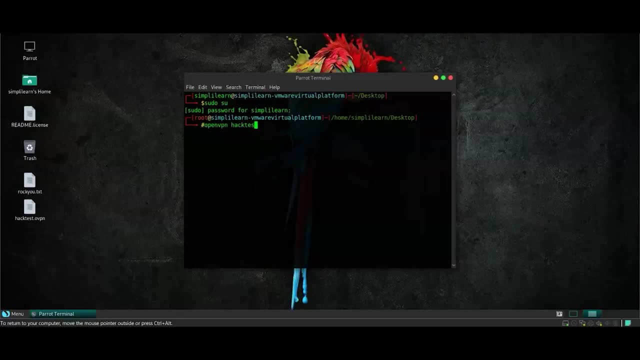 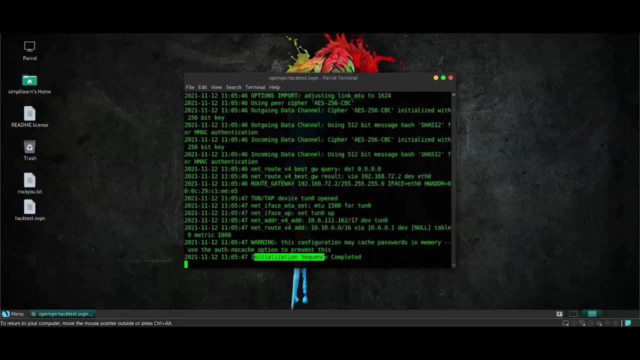 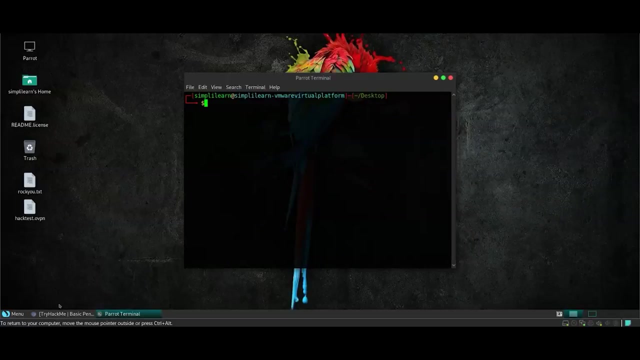 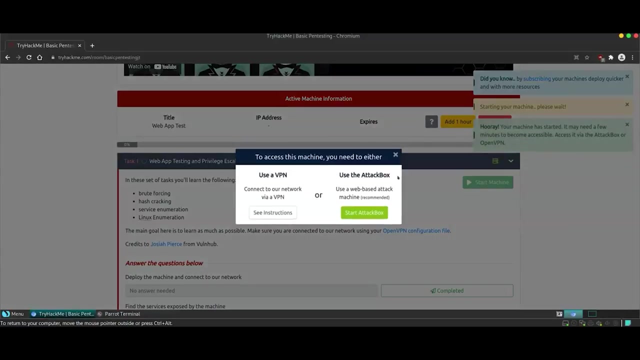 and we're going to connect to it hacktestovpn. Once we see the message initiation sequence completed, we can be sure that we have connected to the network which has the vulnerable machine. Now to start the vulnerable machine, you're going to click this button and wait for a few seconds. 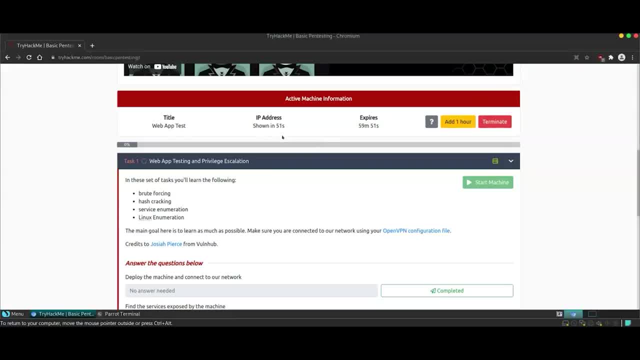 As you can see, it gives a one minute countdown before it shows you the IP address. Now, remember, whatever the IP address we receive here, it is a machine being launched on the TryHackMe servers, But we can connect it to the network by using the network which has the. 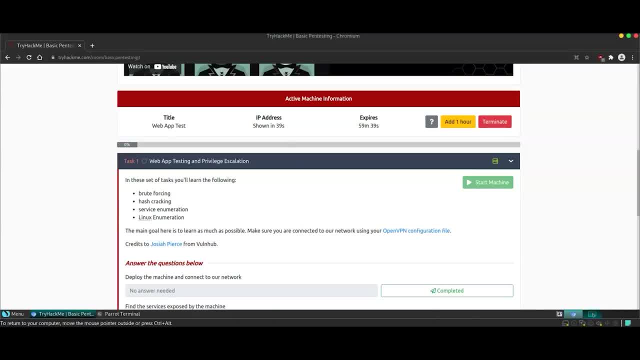 can access that machine because of the ovpn connection that we have just set up using this file. this ovpn file can be found on the tryhackme servers profile section, which i downloaded beforehand. as you can see, we now have the ip address of our victim machine. let's try if we. 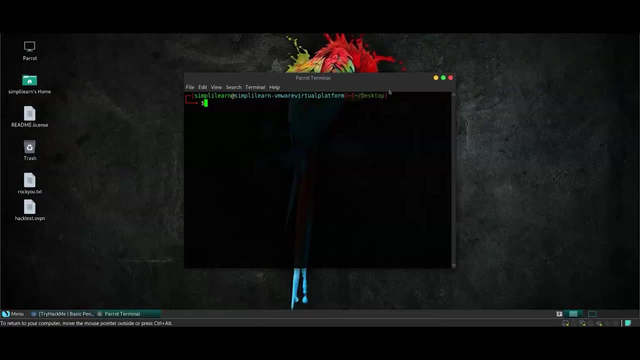 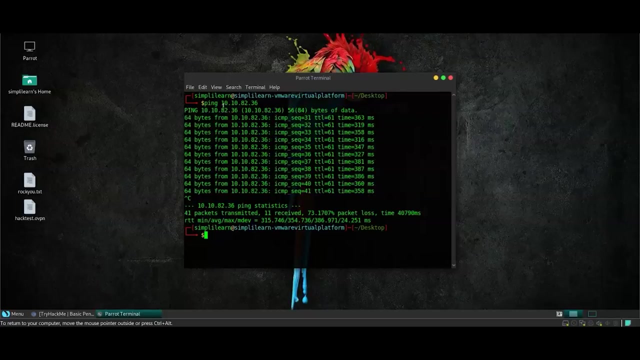 can reach this machine or not. we're going to copy the ip address and we're going to try and ping to the machine. if the connection is successful and we have joined the network, we should be able to see some response over here. as you can see, we're receiving request pings from the victim machine. 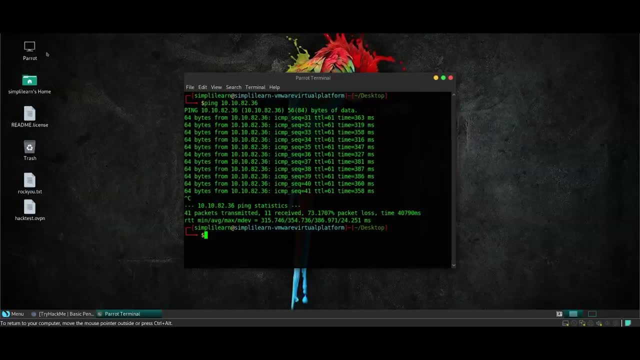 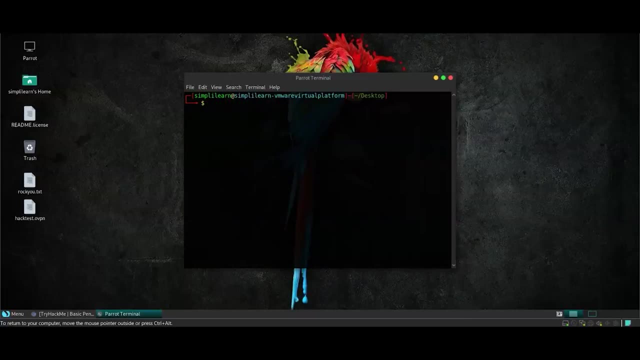 which means that we have already joined the victim network. you, now that we are confirmed, we are able to access the available machine. let's run the first step in a penetration test, which is reconnaissance. let's run up and map scan. we're going to use the flag of sv so that we can know which version of the service it is running. 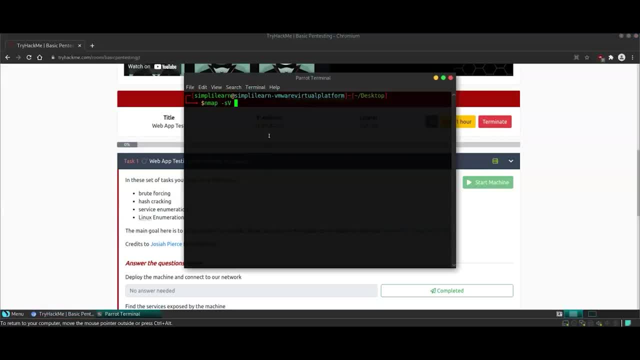 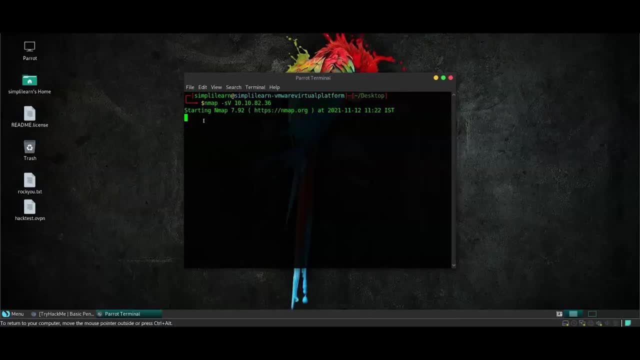 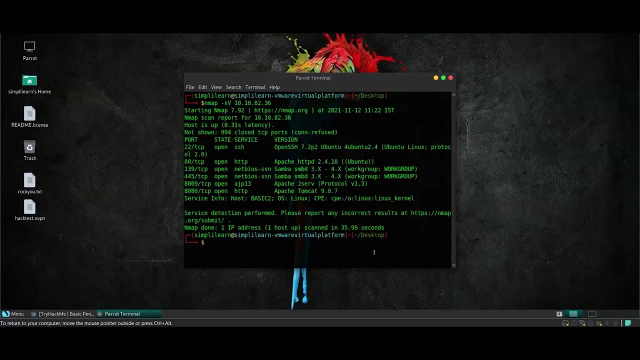 we're going to take up the ip address and paste it here. this scan will only be possible if the openvpn connection is up and running. as you can see, it is still running and we have a results over here. by running the scan so that we can find the services running on the host machine that we will run and map against, we conclude that. 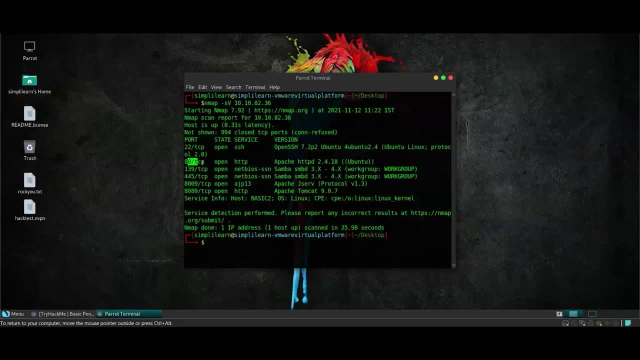 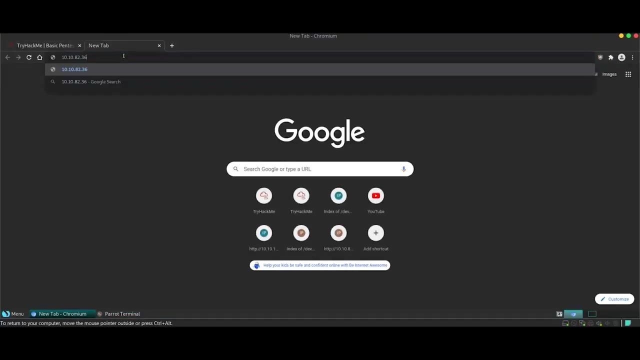 a web service is running actually on port 80, as we can see over here, which is using the apache server system. novamente addition to this, there is a SMB Samba service as well, running on ports 139- 445. now that we know they have an Apache server, we can use this IP address to. 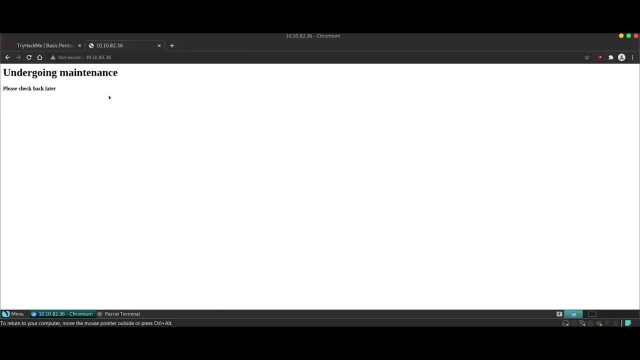 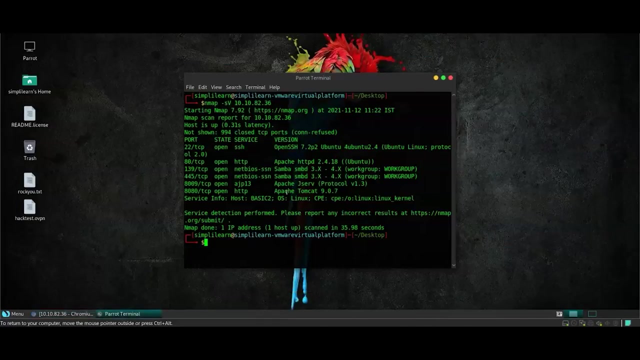 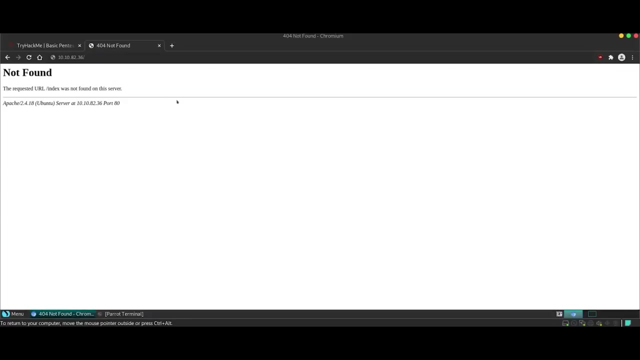 open it on the browser. okay, since the current home page is not accessible, we can use some other URLs as well. as far as Apache servers are concerned, there are a certain set of URLs that can be used to open. however, if we go to the URL, which is IP address, slash development, this opens up a new folder. if we try to. 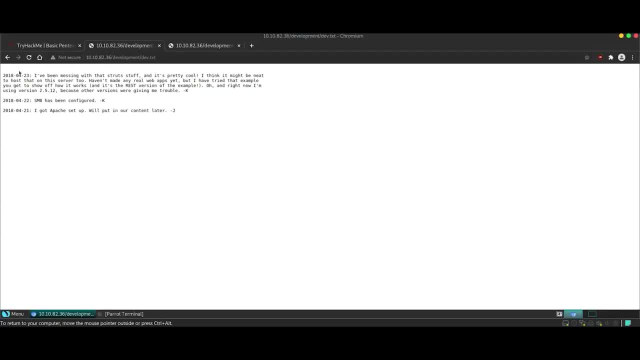 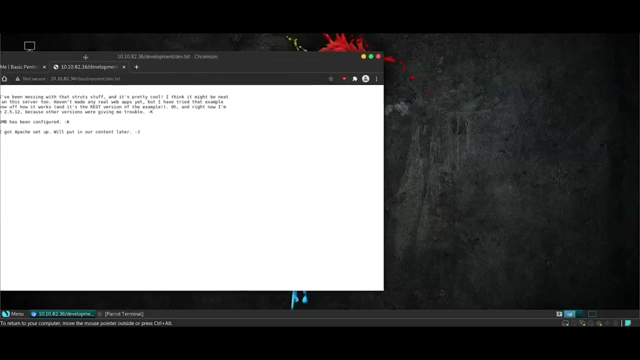 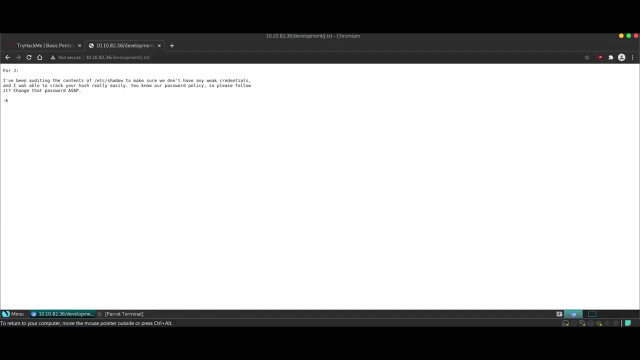 check the contents of these files. this is for the dev dot txt. you can see the version of the Apache HTTP server that is being run. this is the dev dot text. if we go back and we check the second file as well, it says the contents. the shadow has the credentials. 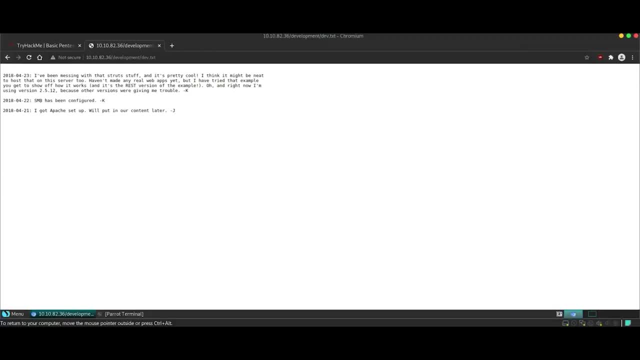 okay, if we go back to the server, we can see that the contents of these files are the same as before. so if we go back again, SMB has been configured, which we have already found out, and map that it is running a Samba server now with this. 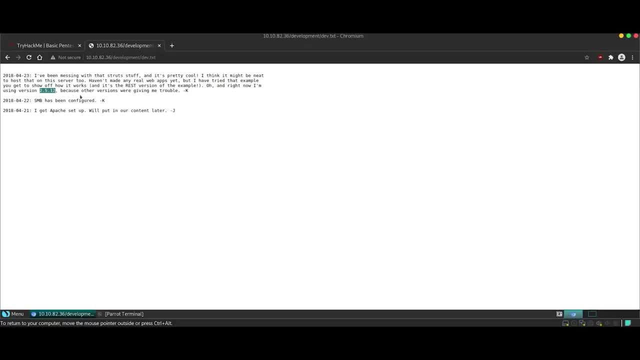 version of the Apache server. we can find version specific exploits that can be run on Metasploit, but there is sometimes no, no need of that. we can use another technique. as we now know that there are multiple users that is being run over here. we can use a tool known as enum for Linux. 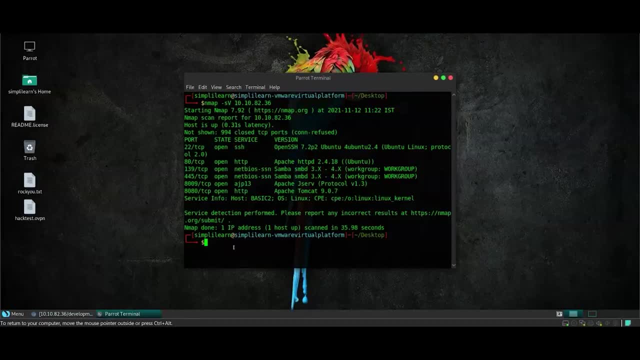 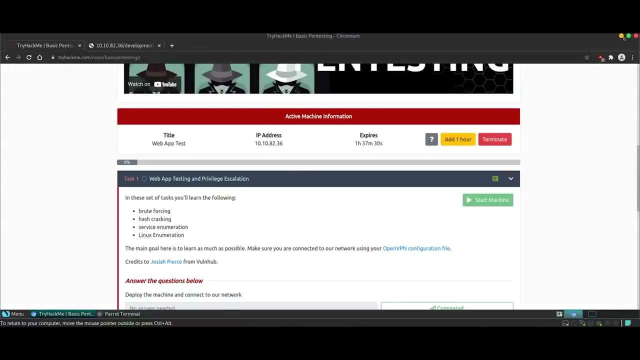 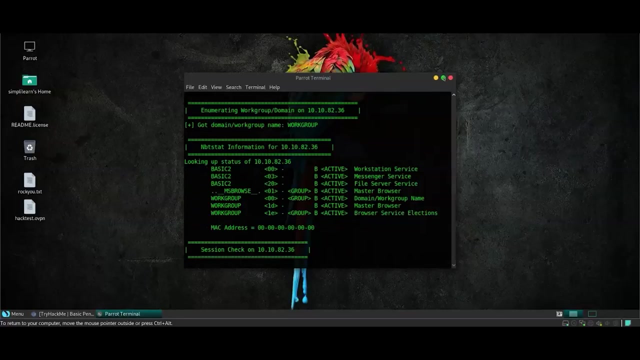 what it does? this is acts at enumerates the windows and a Samba systems to run that command. we're going to use enum for Linux minus a and we're going to take IP address of the machine paste it here. what this will essentially do is provide us usernames that are being stored in the vstack server. 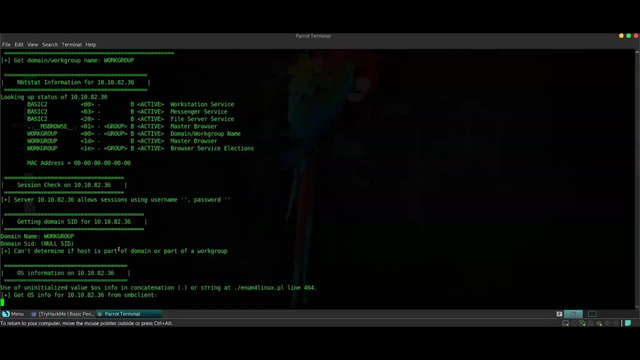 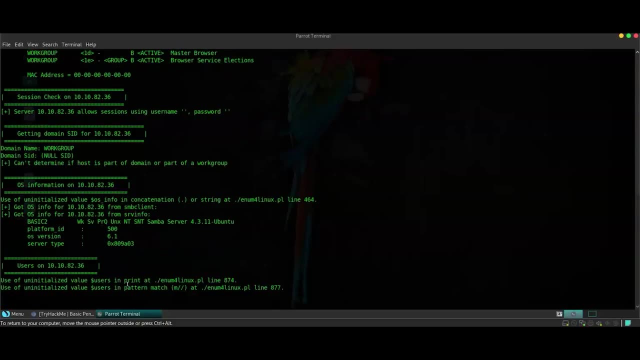 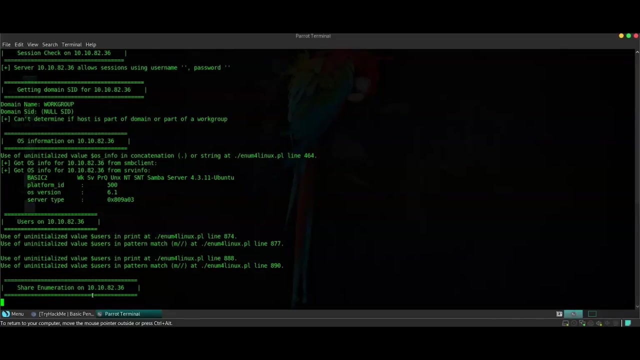 in the victim machine. it's going to take some time to find out the usernames. once you find those out, we can run the necessary attacks. as we have already seen on the n-map, it is also happening in SSH port. so if you find the username and we find a single hash that can be cracked, we can use the SSH to get inside. 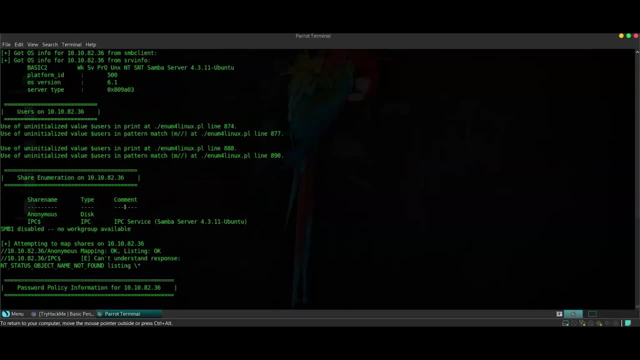 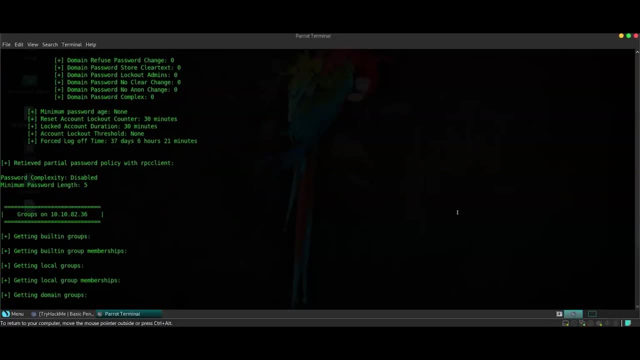 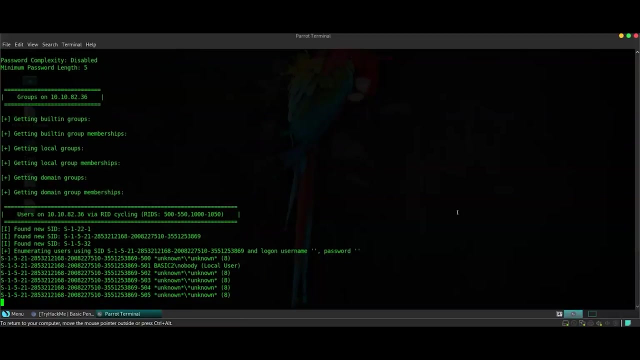 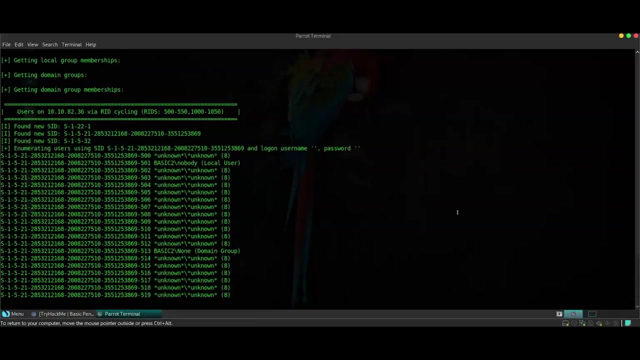 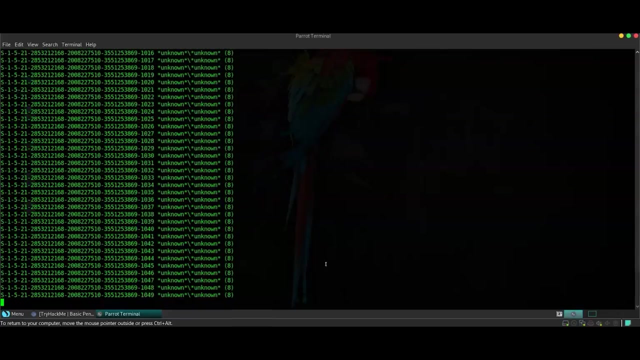 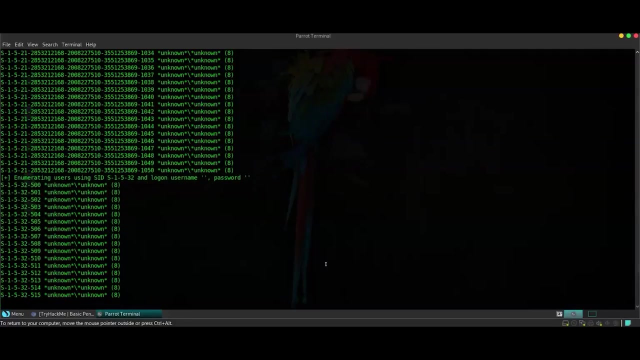 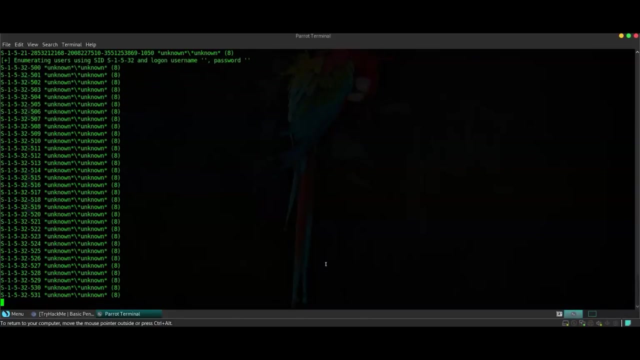 the machine. right now we have to wait for the results of the enum for Linux command and we'll see what happens. as you can see, We have found two users of the machine known as K and Jan. I think we can stop the enumeration right now, since we have the two users of this machine. 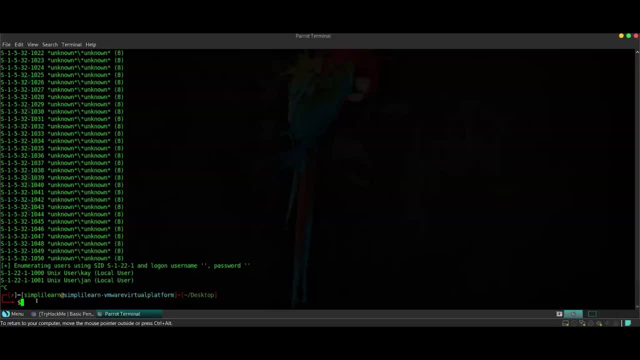 Next step. what we can do is we can try to SSH into the machine. Now, to run the SSH command, we're going to need the password of one of the users. For this example, let's say we go with the user of this machine. 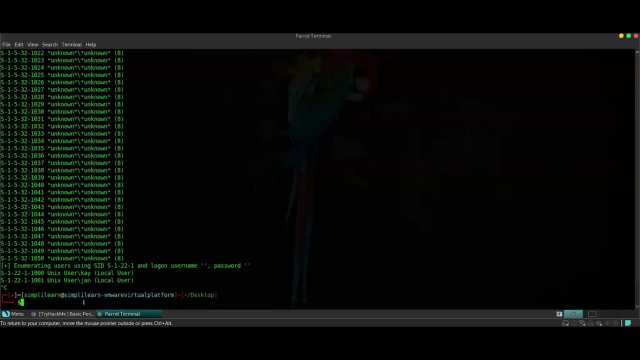 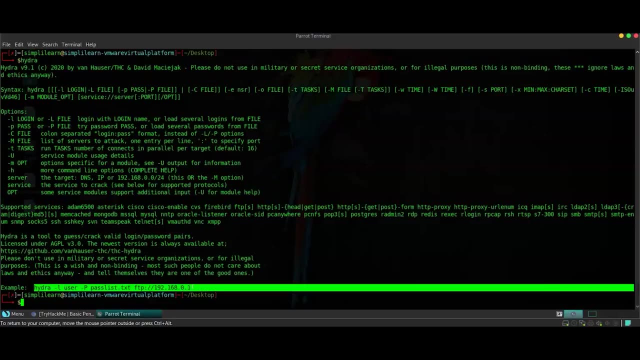 Jan To brute force. we're going to use the Hydra tool like an example command. This is how we can use. Let me just copy this and paste it over here. Alright, Hydra minus L User. as we have already decided, we're going to use the user Jan and. 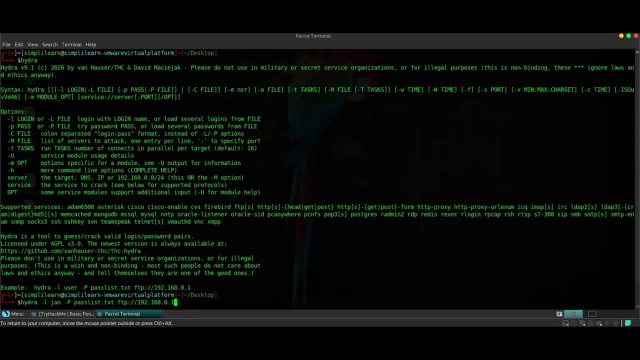 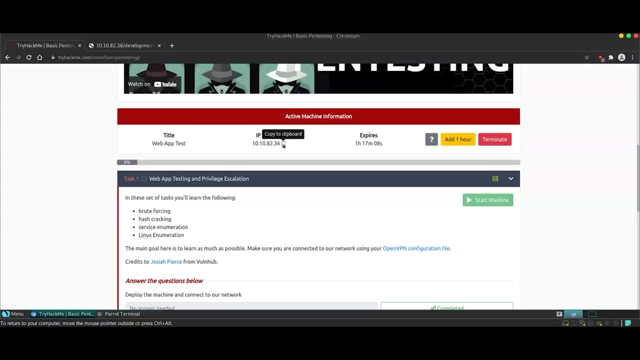 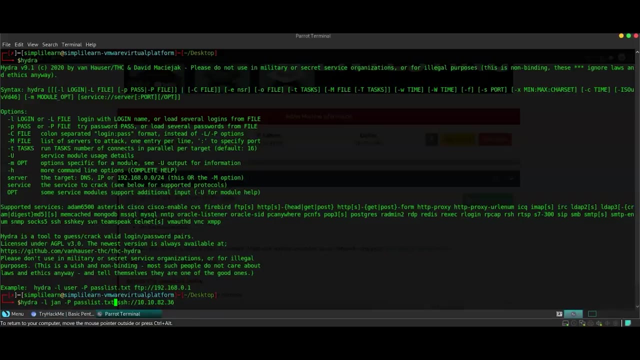 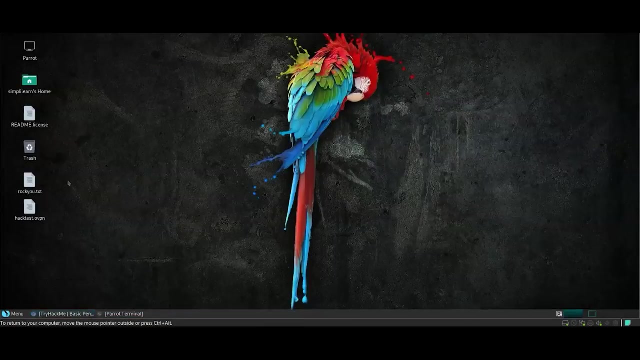 we're going to use SSH For the IP address. we're going to copy it from here and paste it here. Now for a password list. we're going to use a word list which has a few passwords already present in it. For this example, I'm going to use the rockutxt file, which has millions of passwords already. 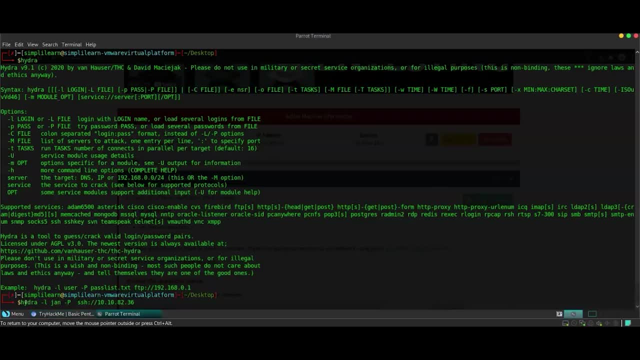 stored in it What The Hydra will do. ogniberry coisa To construct Ver explanation here. there is some work with that line right now. to� To create will try to bypass the SSH console on the machine using the passwords present. 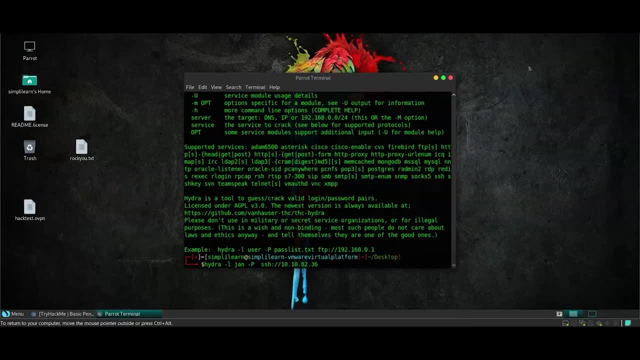 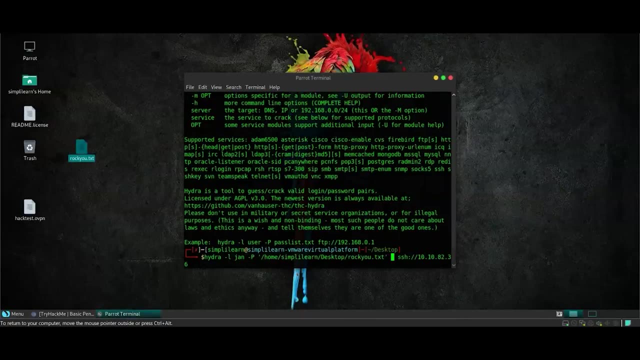 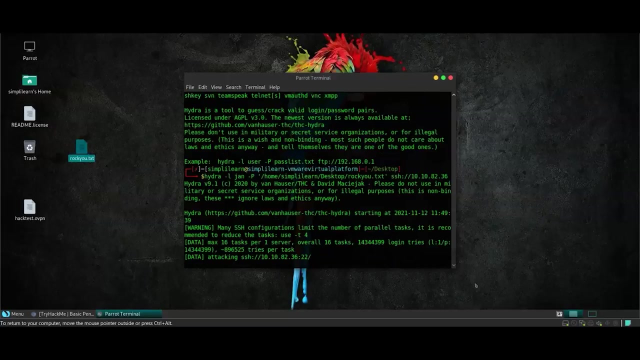 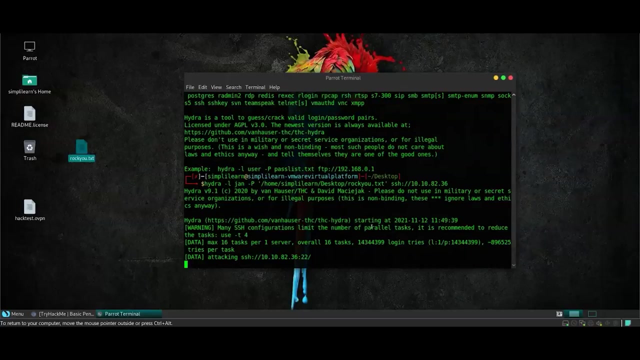 in the rock you dot txt file. we will give the path rock you over here like this, and we're going to run it. as you can see, it's mentioned that it's attacking SSH at this IP address. now this attack is going to take a while and after this attack is done, we are going. 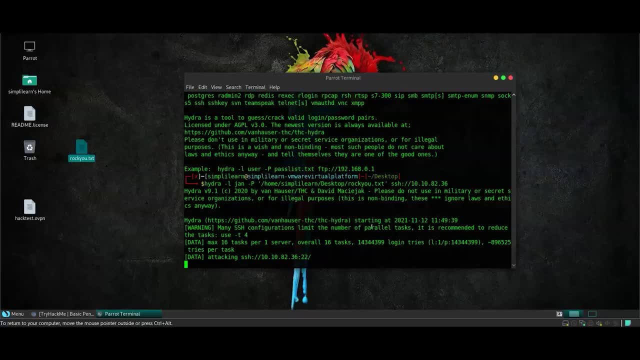 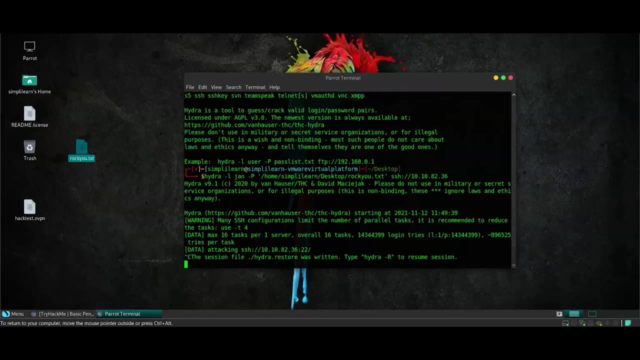 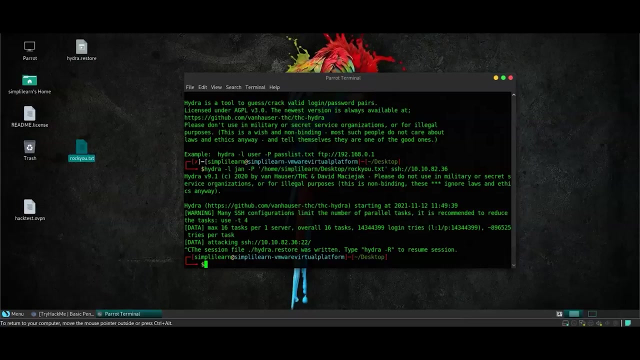 to get the SSH password, which is basically the credentials of the Jan user in the victim machine. for now, I'm going to stop this attack, but I would recommend is for you to run this attack and write down the password that you received in the comment section below the password. 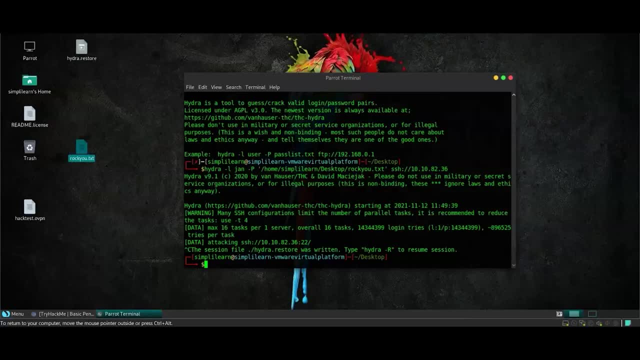 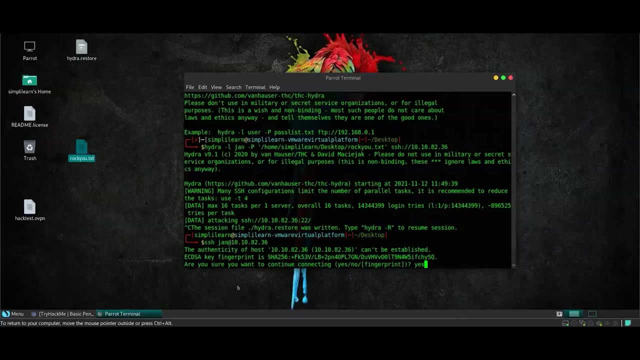 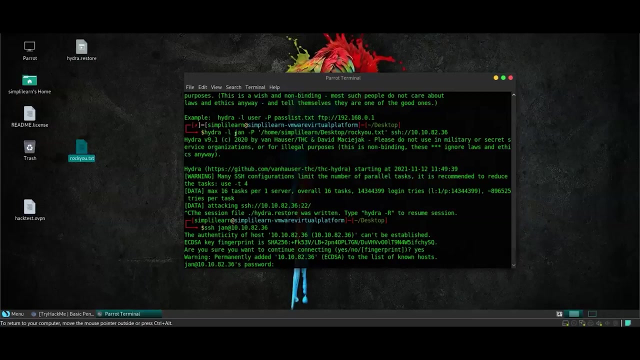 that we receive from here can be used to log in into the machine. let's try that once. to SSH into the machine, we're going to write SSH user at the rate IP address. we're going to write yes and press enter. now we're going to enter the password that we have found after running the 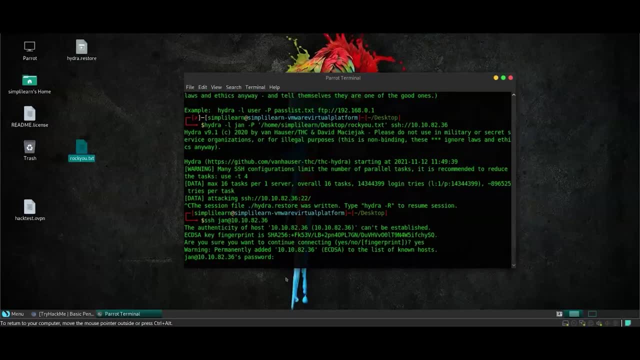 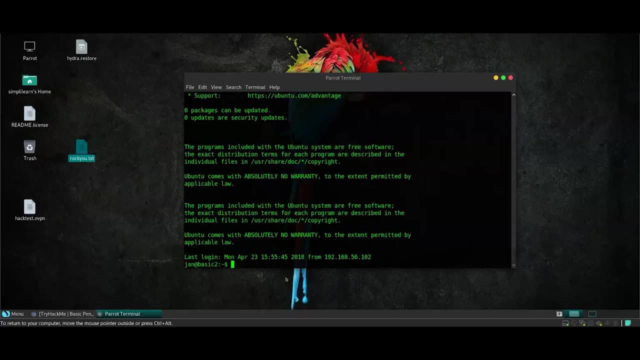 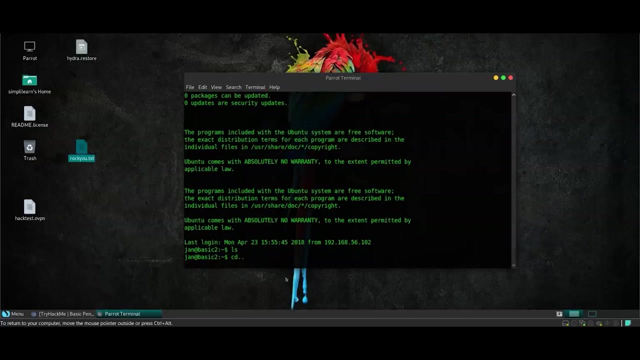 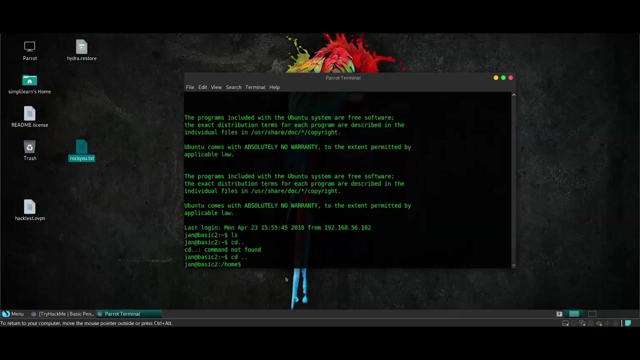 Hydra command. I'm going to type the password and press enter and we have logged in, as you can see. now, if we try to look around, there are no directories over here. okay, so let's go one step back, give a space over here. okay, let's go to the second users folder. 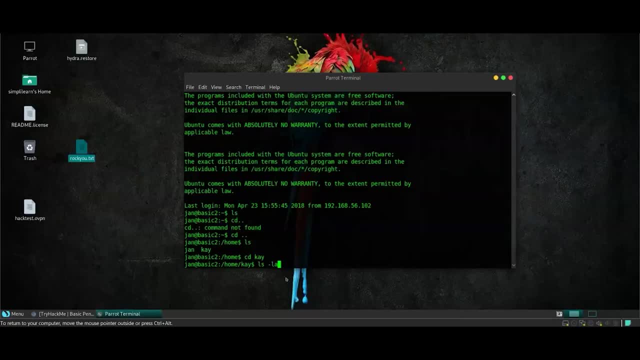 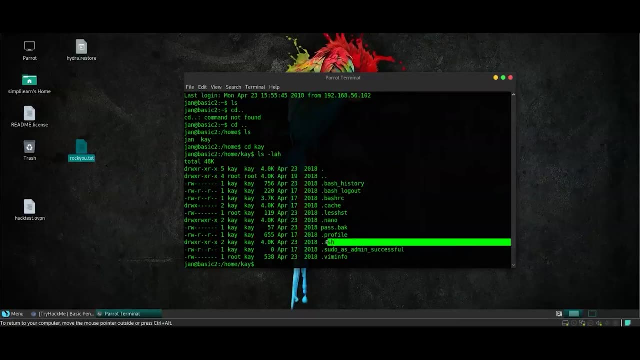 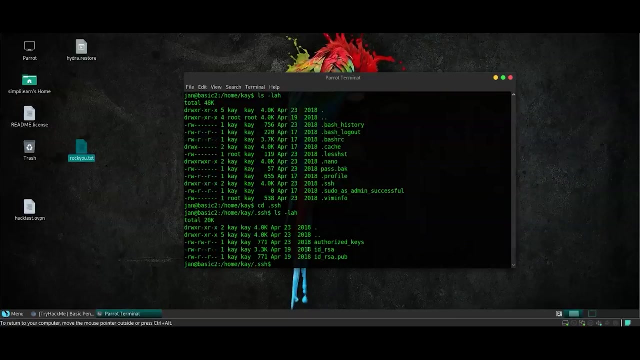 okay, these are the contents of the K folder and you can see there's a dot SSH folder over here, so we're going to enter that. let's have a look: the files in this folder and we can file in RSA ID over here, which, if I'm not wrong, should be an RSA private key. 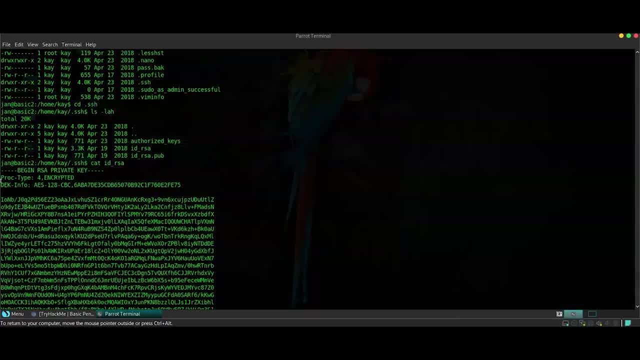 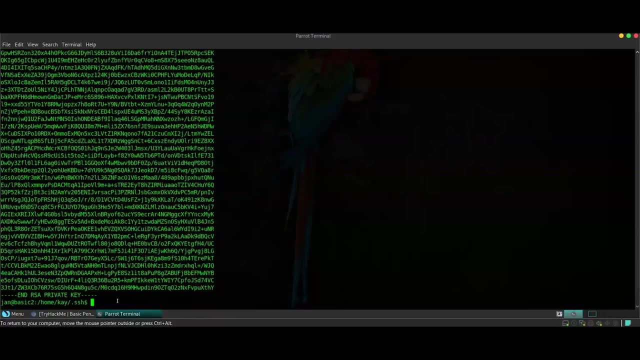 which can be used to SSH into the machine. here we go. you can see it's a big in RSA private key and it should end here as well. now what this private key does. this hash will be used to log SSH into the machine when using the user K. 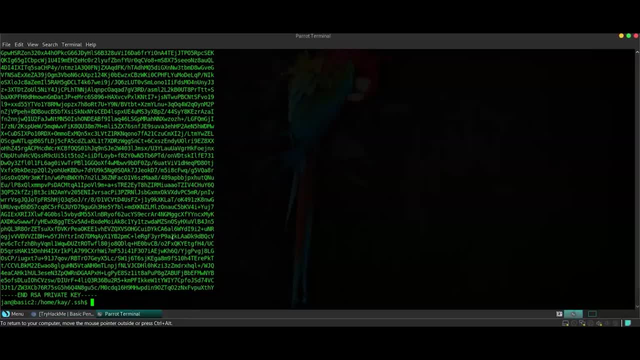 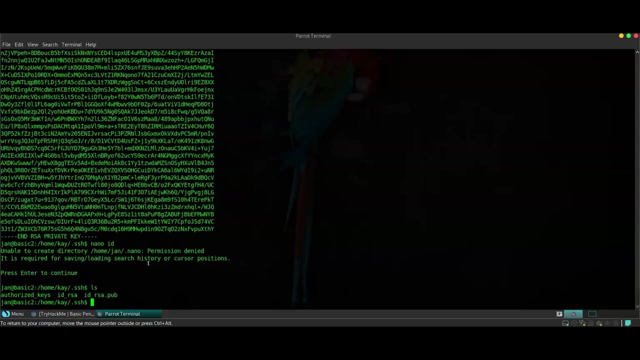 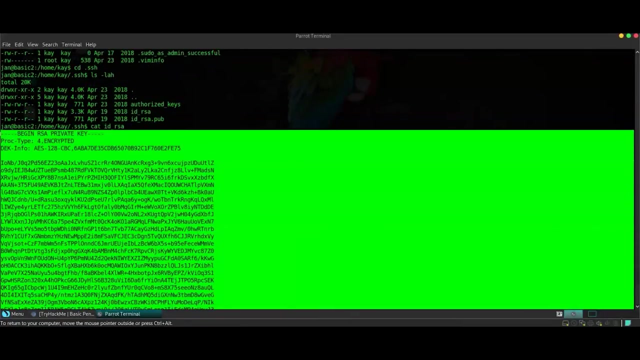 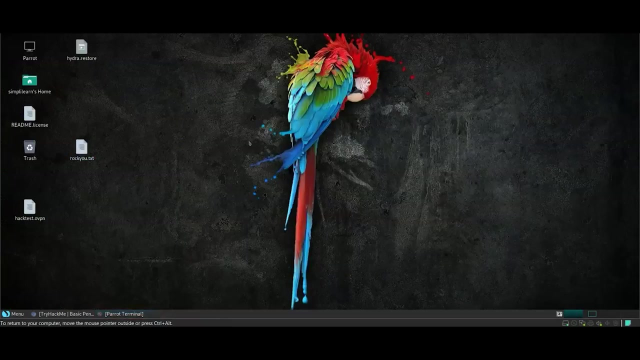 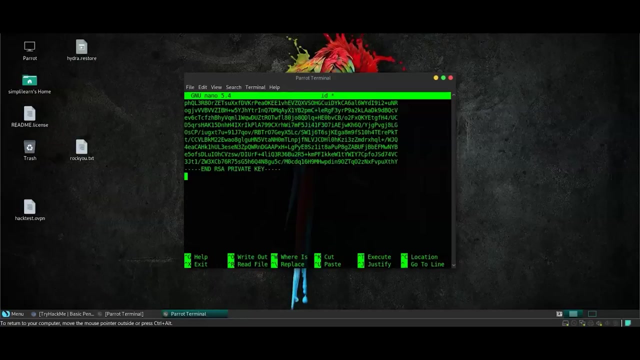 once this hash is cracked using Hydra or any other cracking software like John the Ripper, we can easily use the passphrase to login into the machine with the user of K. what I am going to do is copy this private key. you launch a new terminal, create a new file known as nano ID, paste the private key. 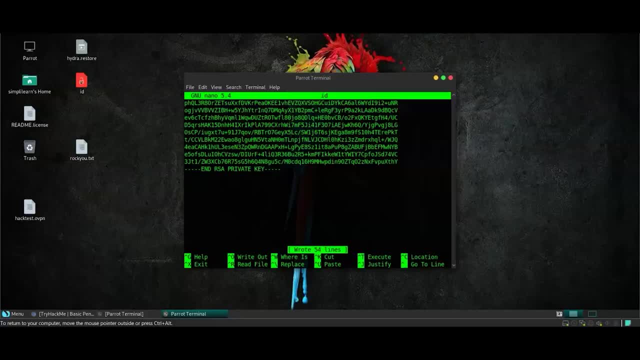 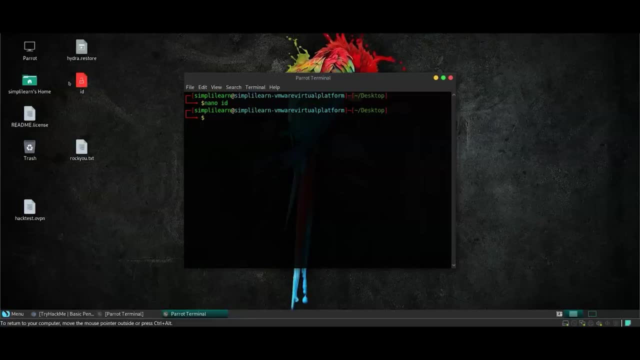 over here and save it. as you can see, you have saved the file over here now. this hash can later be used to crack into the machine using the user of K. this hash can be cracked using either John the Ripper, Hydra or there are other cloud mechanisms that can be used to crack this machine. after it is cracked, we can. 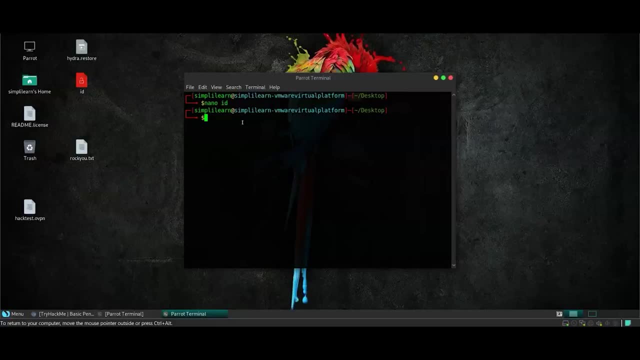 use the passphrase derived from it to SSH into the machine to perform the SSH entry. we're going to use this command: SSH minus I. we're going to use the same file which we received. we're going to write the user name, which is K 10.10. we can just copy it from the here right, minimize this and paste the. 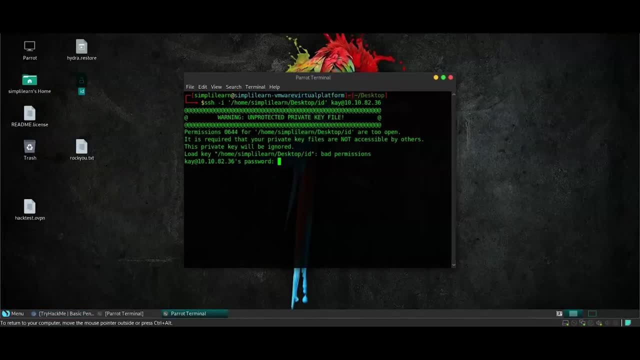 IP address over here, or we can do one more thing. we're going to use a sudo command together as well. it's better: sudo SSH. enter the system password. this passphrase is the one that we received after cracking the hash in this ID file. whichever password you received after, 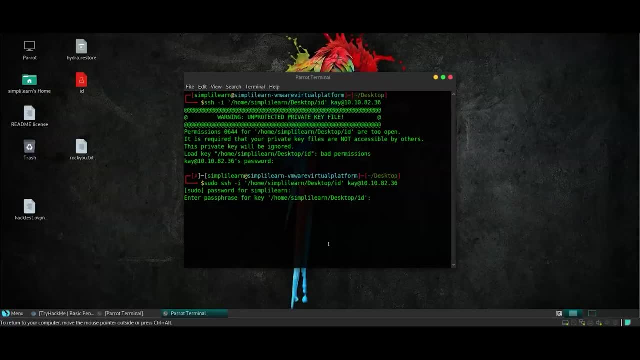 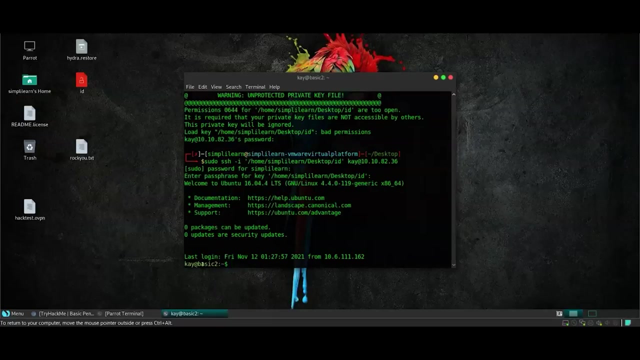 cracking this using Hydra or John the Ripper. please write the password in the comment section so that we can know that we have successfully cracked the hash in the machine. the password: we're going to write the passphrase over here, press enter and, as you can see, we have entered the system of K here. we're going to press LS and we 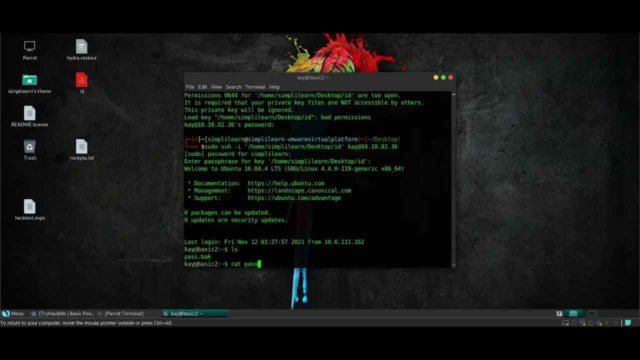 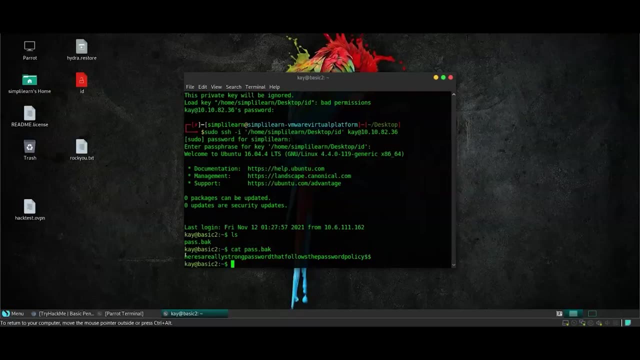 find the backup file of the password. we're going to write cat password back and here is the final root password. so, as you can see, we have now able. we have now received the final root password of the primary user and we have already cracked the password of the other user, that is Jan. so this is the 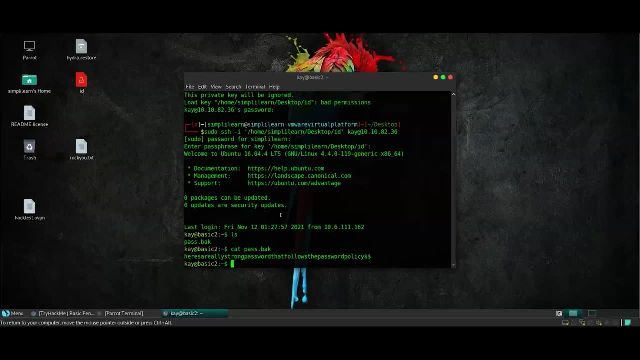 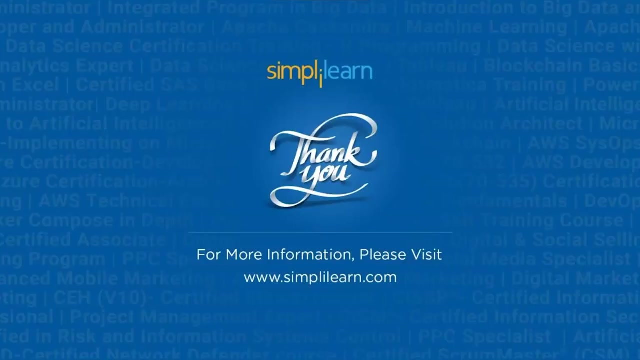 entire process of how you can use nmap to find out the valuable points. you can see which other software's that are running, which versions they are running and which of those versions have a legitimate claim as an insecure exploit. hope you learned something new today. if you have any questions regarding the 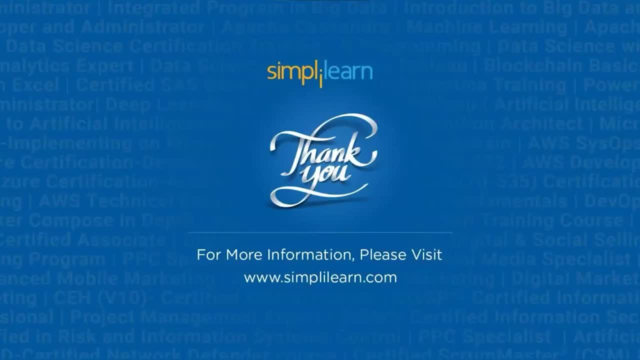 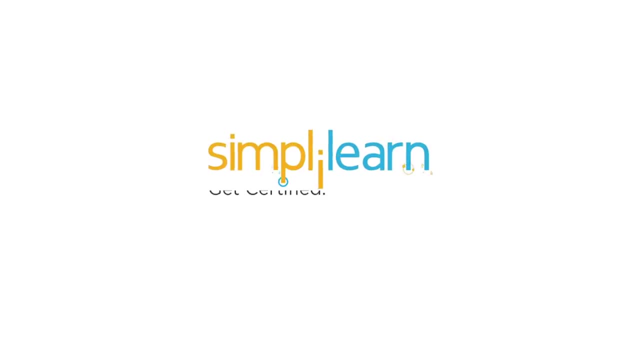 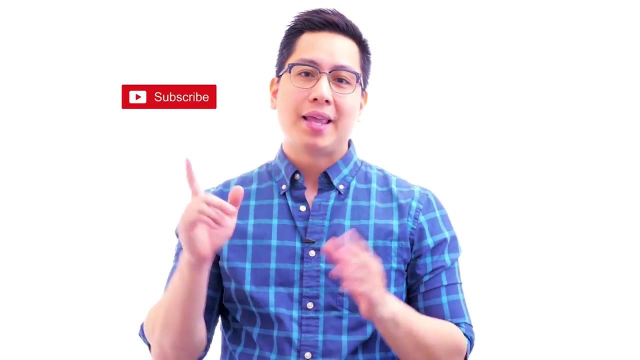 topic. please let us know in the comment section below and we will get back to you as soon as possible with the solution. subscribe to our channel for more informative videos and thanks for watching hi there. if you liked this video, subscribe to the simply learn YouTube channel and click here to watch similar videos, to nerd up and get certified. click here.